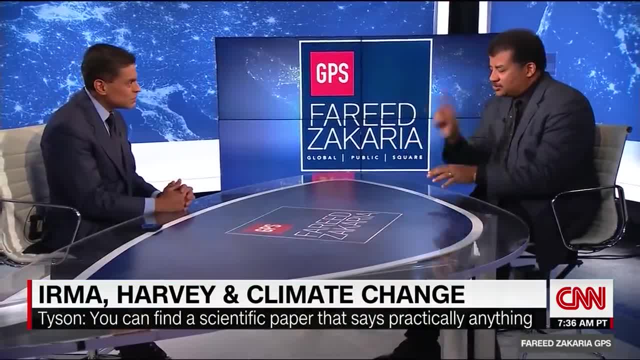 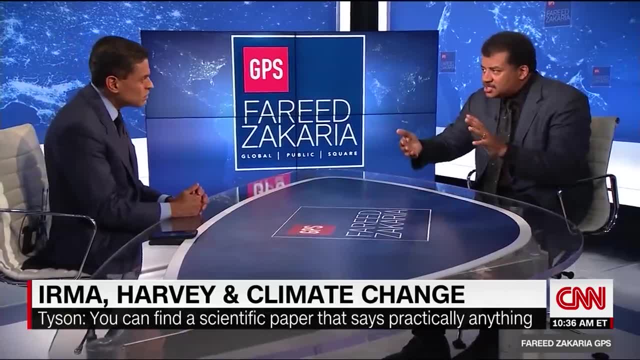 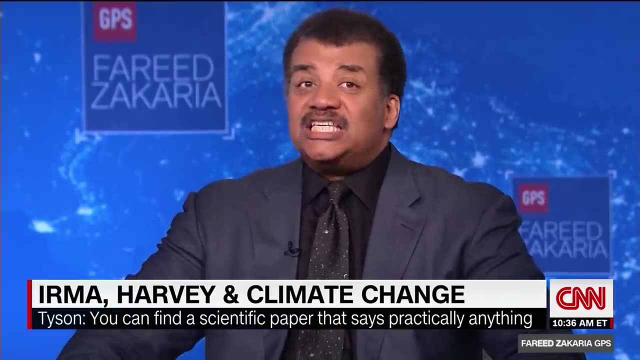 a truth that is true, whether or not you believe in it. it requires more than one scientific paper. It requires a whole system of people's research, all leaning in the same direction, all pointing to the same consequences. That's what we have with climate change as induced by human conduct. 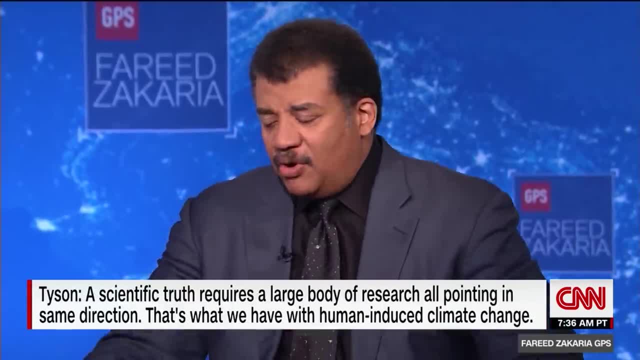 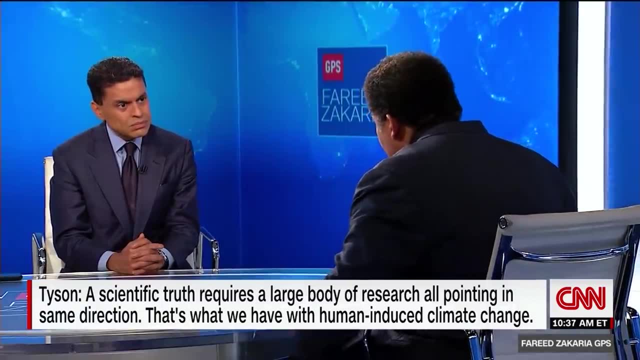 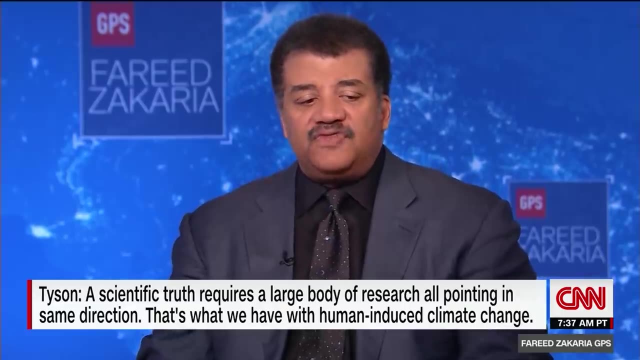 This is a known correspondence. If you want to find the 3 percent of the papers or the 1 percent of the papers that conflicted with this and build policy on that, that is simply irresponsible. And how else do you establish a scientific truth if not by looking at the consensus of scientific experiments and scientific observations? 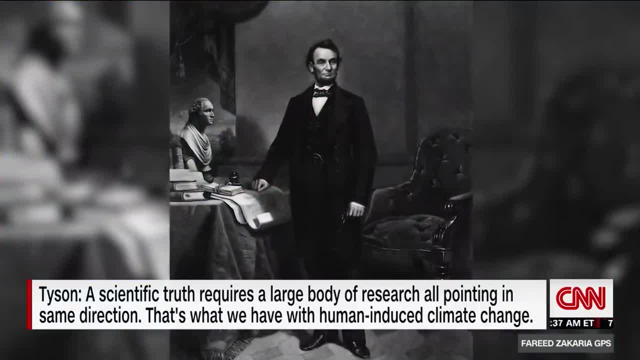 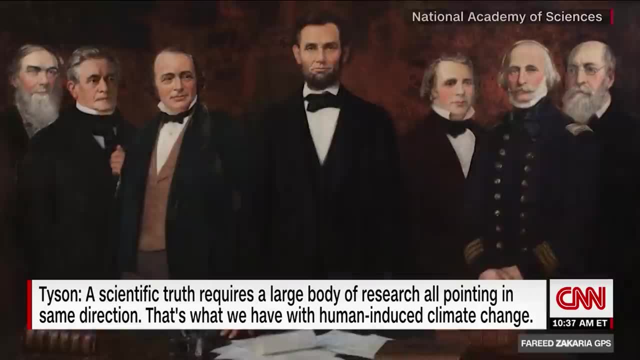 Abraham Lincoln, the first Republican president, signed into law in 1963, a year when he had important things to be thinking about Right. He signed into law the National Academy of Sciences because he knew that science mattered and should matter in governance. 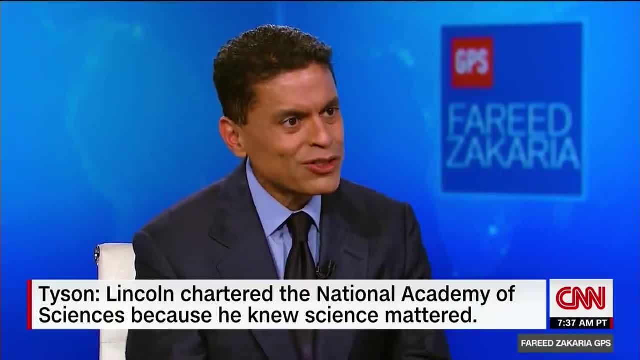 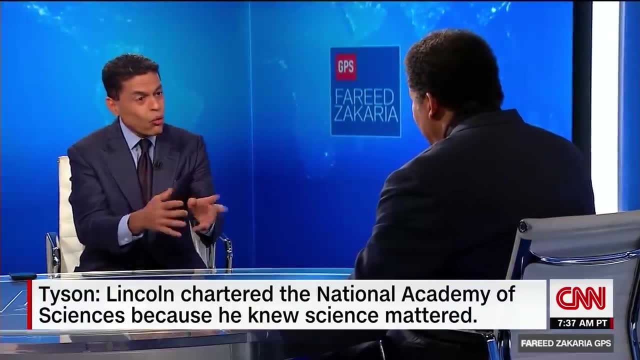 And you know, we build our cities on the basis of science. When we fall ill, we don't go to the local witch doctor Right, We go to a doctor, Even though all of that science is still. you know. I mean, there are advances going to be made. 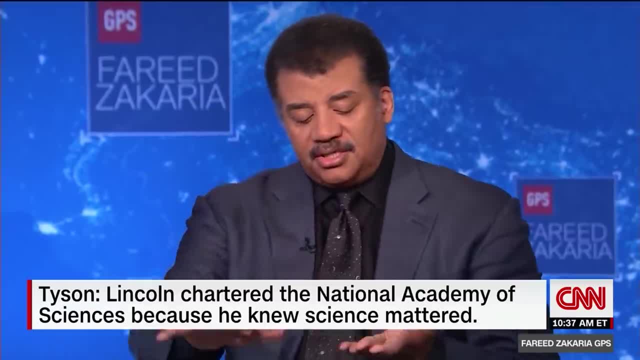 None of it is settled in the sense that, Well, so you know it is settled, You know it is settled. Settled science is the science that has come out of large bodies, Right, Large bodies of research that all agree, Right. 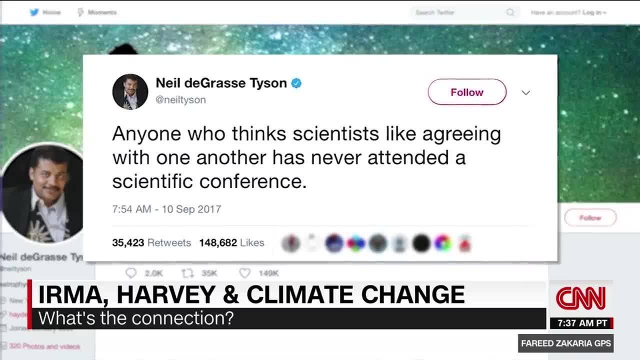 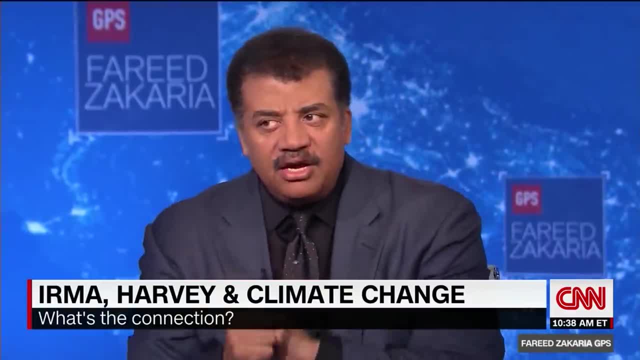 When you see scientists arguing- and I tweeted- I said: if you think scientists want to always agree with one another, you've never been to a scientific conference because people are duking it out. But what are they fighting over? Not the settled science that's been in the books. 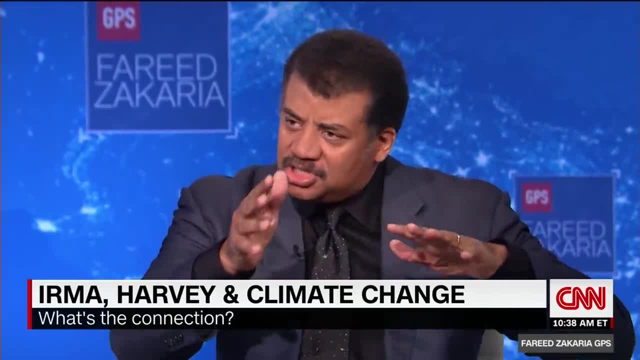 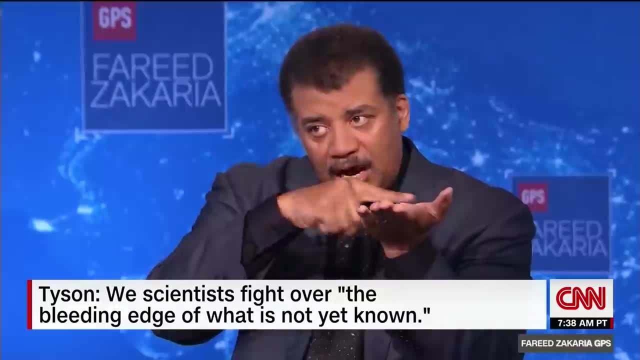 We're fighting over the bleeding edge of what is not yet known, And that is the natural course of science. Now, if you, as a journalist, want to eavesdrop on that meeting, you'll think scientists don't know anything about anything. 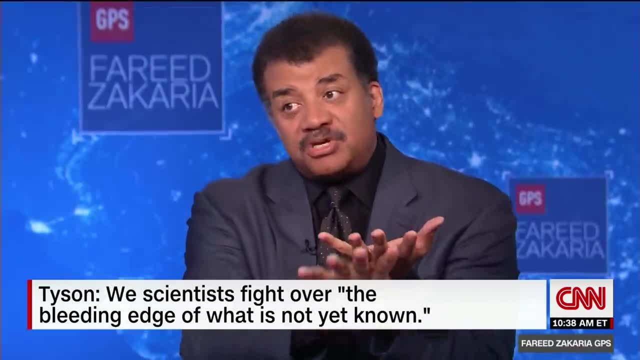 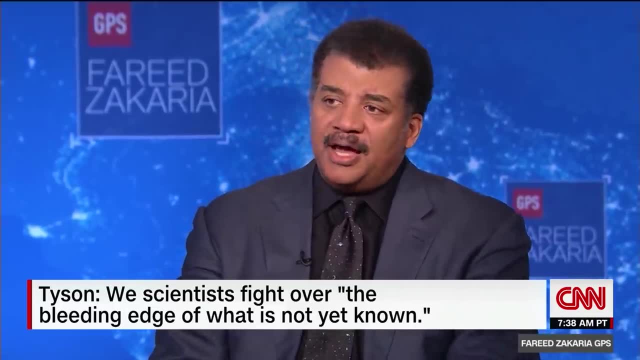 But it's the body of knowledge that is accumulated over the decades that precedes this that becomes the canon of what. if you're going to base policy and legislation on, that's what you should be thinking about. So you would say this is a moment to listen to climate science. 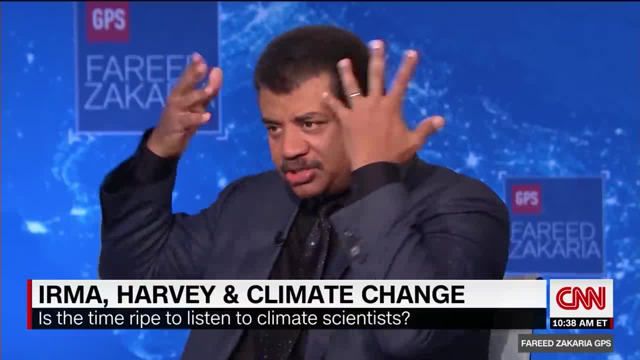 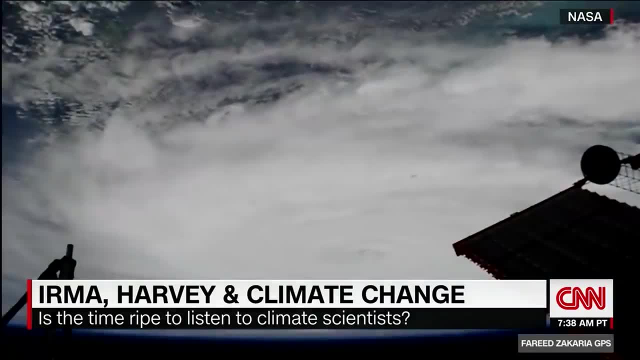 I think there's 50 inches of. I can't even picture how many raindrops. is that 50 inches of rain in Houston? This is a shot across our bow, A hurricane the width of Florida going up the center of Florida. 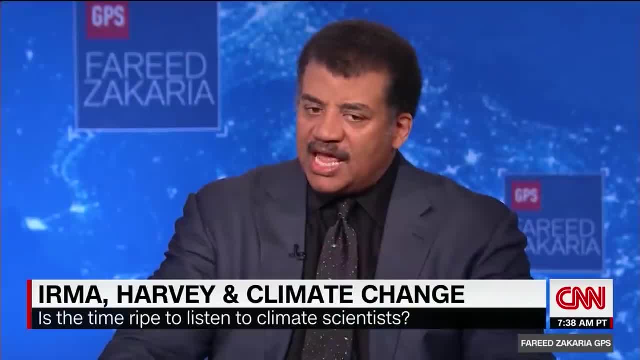 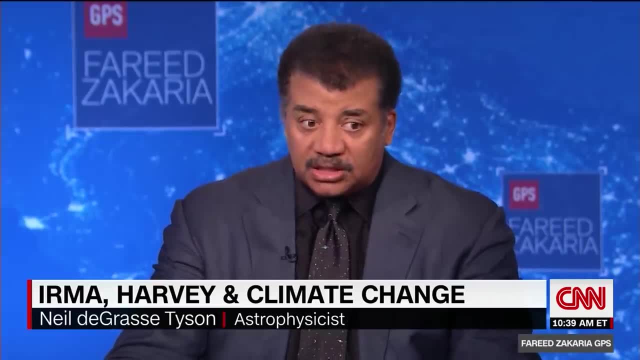 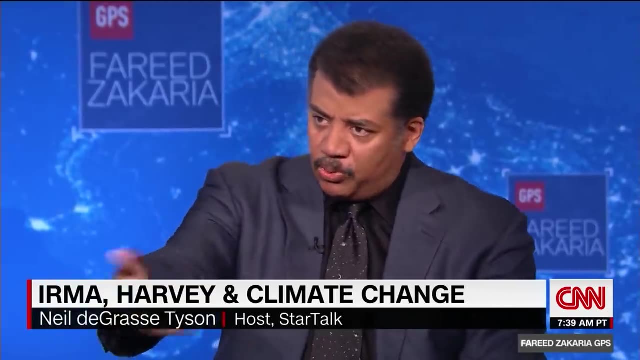 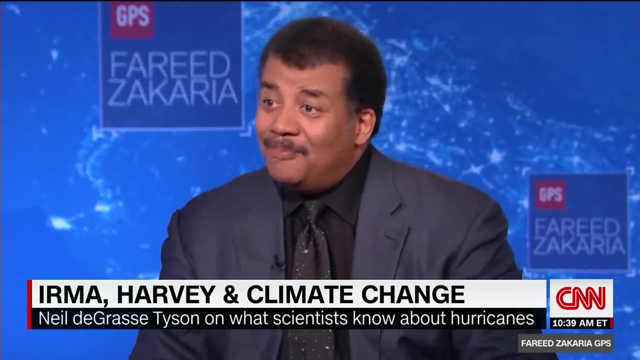 These are. These are shots across our bow. What will it take for people to recognize that a community of scientists are learning objective truths about the natural world and that you can benefit from knowing about it? Even news reports on this channel talked about the fact that we have fewer deaths per hurricane. 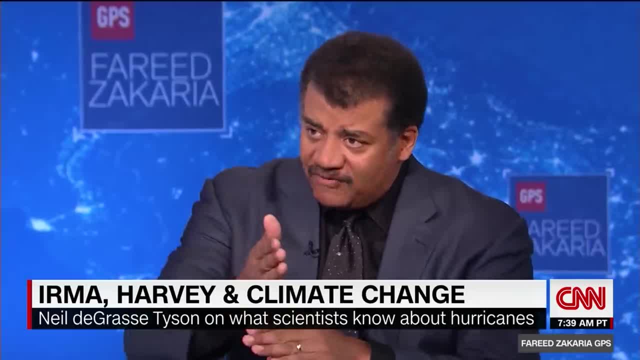 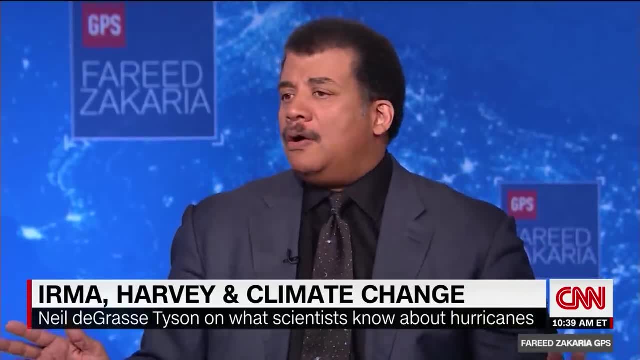 Why? Because you now know weeks in advance. We have models that have trajectories of hurricanes In decades gone by. it was like there's a hurricane there, we don't know: should I stay, should I go? And then you stay and you die okay. 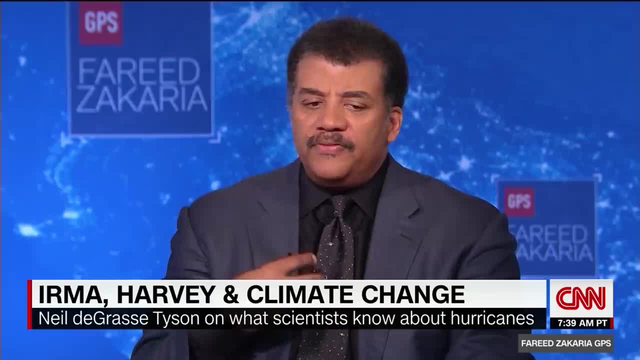 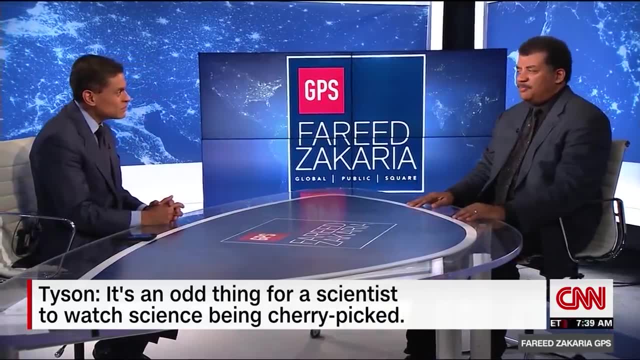 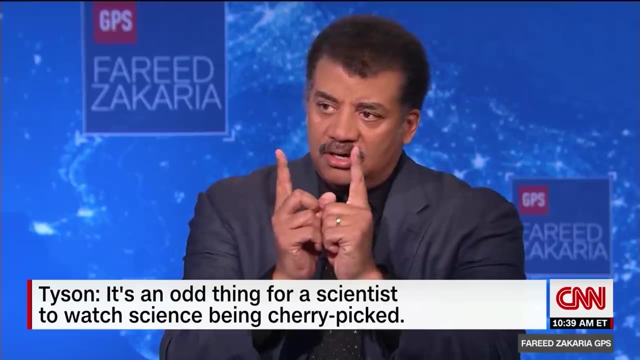 So to cherry pick science? it's an odd thing for a scientist to observe, And I didn't grow up in a country where that was a common phenomenon. We went to the moon and people knew science and technology fed those discoveries. And the day two politicians are arguing about whether science is true. 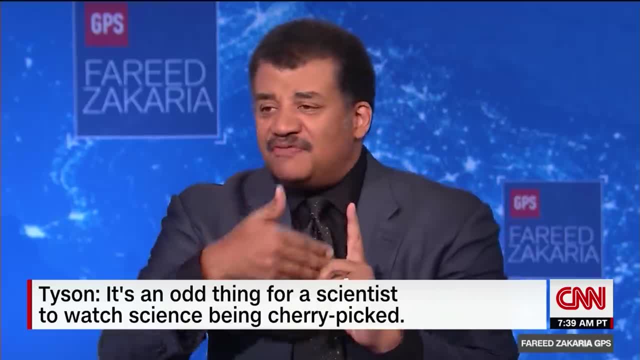 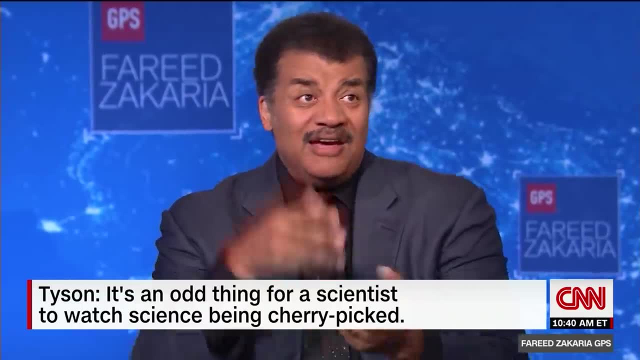 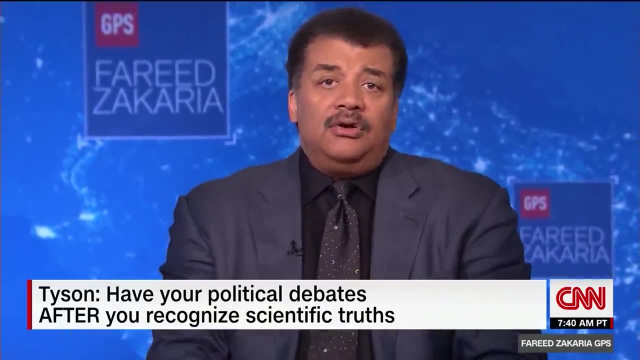 it means nothing gets done. Nothing, It's the beginning of the end of an informed democracy. as I've said many times, What I'd rather happen is you recognize what is scientifically truth, then you have your political debate. So, in the case of energy policy, whatever you don't ask is the science right. 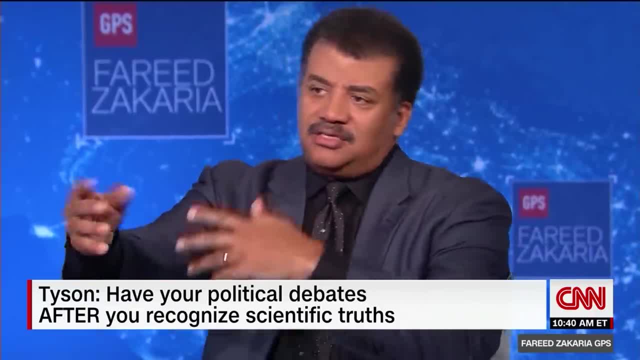 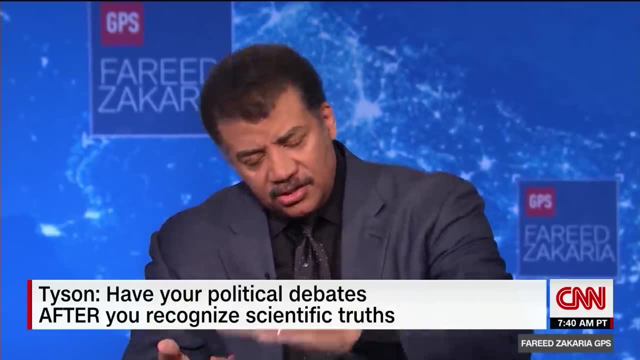 You ask: should we have carbon credits or tariffs? What's the right response Exactly? What is the economic dimension of this? That's where the politics, The economy, has come to a point where people are like it needs to come in and it's not. 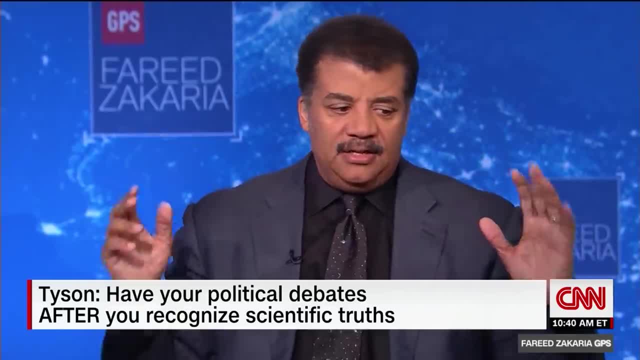 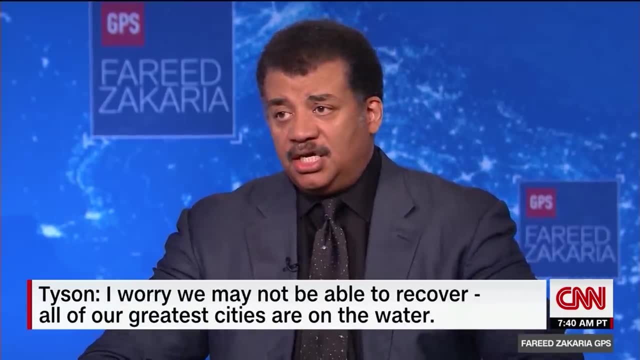 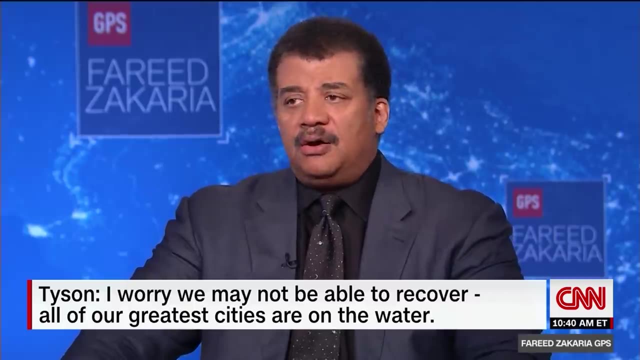 The longer we delay, the more I worry that we might not be able to recover from this, because all our greatest cities are on the oceans and water's edges, historically for commerce and transportation, And as storms kick in, as water levels rise, they are the first to go. 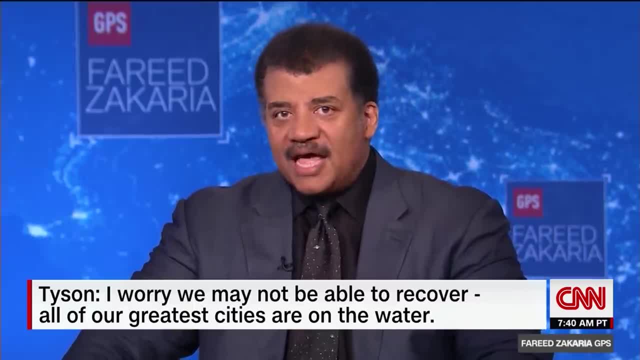 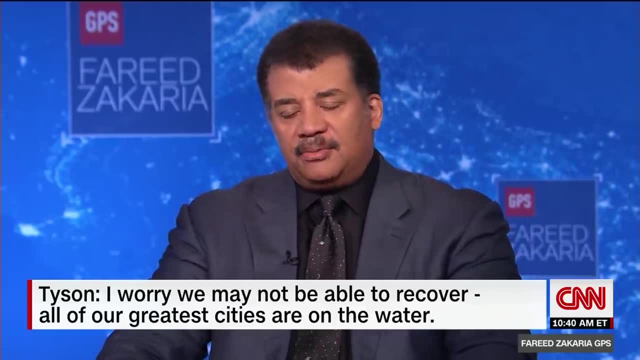 And we don't have a system, We don't have a civilization with the capacity to pick up a city and move it inland 20 miles. This is happening faster than our ability to respond. That could have huge economic impact consequences. On that sobering note, Neil deGrasse, Tyson- always a pleasure And we are in a hurry to. read the book. Thanks,